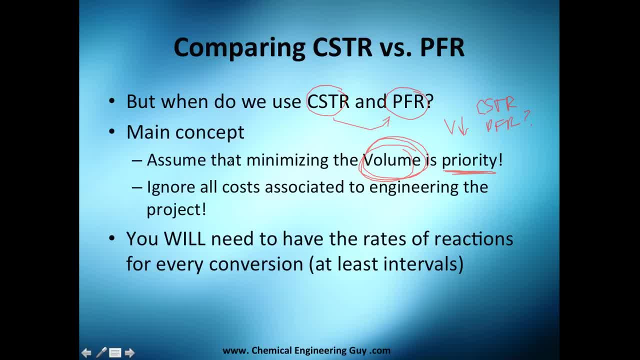 reactor. so that's not nice, especially if you are the engineer. now, ignore all codes associated to engineering. of course you're going to tell me, like now, you need more streams, you need more pumping, you need more a operation cost, whatever. no, we're just going to see right now. volume, let's say volume. 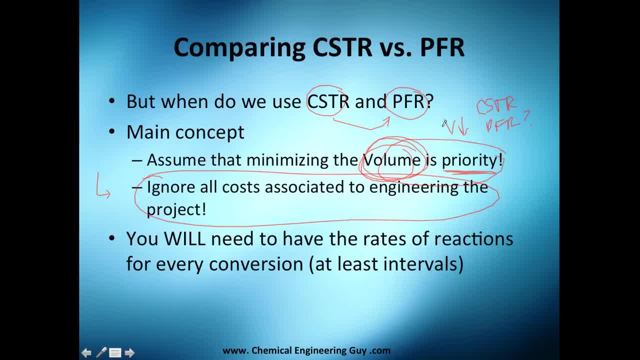 is our priority. let's say we live in a very small plant and it's very hard to grow, which is actually the case for many plants. I remember when I was in Germany there were no space. they got money, but they got no space. so the the priority there was volume, how to get. 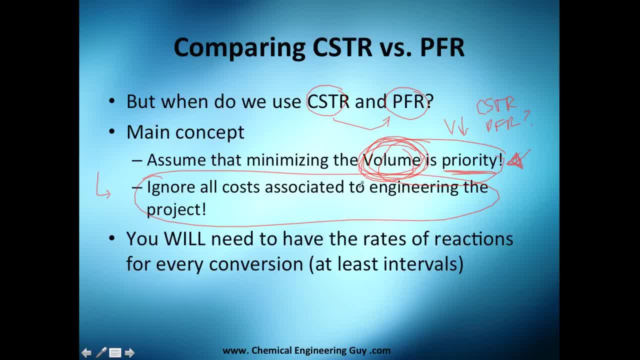 the same reactions in lower or smaller places. so you will need to have the rates of reaction for every conversion. that's true, you're going to have your list and you will need at least various rate of reactions with X. so okay, you can find them, only one will not help. 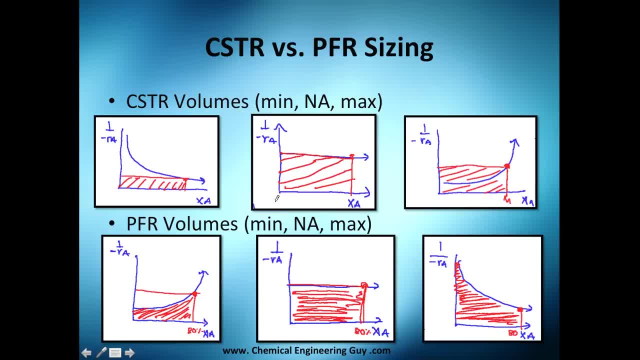 and we've seen this before. probably you're scared because there are two dots, uh, too many here. uh, this is the CSTR. I ordered them from minimum volume to maximum volume. of course, we want to avoid the one in maximum volume. so look, analyze, and I can actually recommend you to pause the. 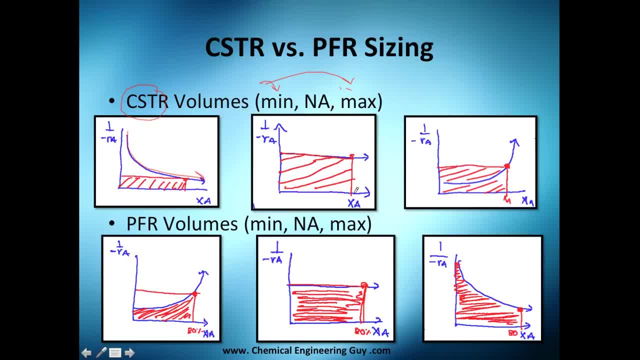 video, try to analyze it for you or yourself and then I explain you. so hopefully you pause it and you saw it, because then I'm going to explain you. okay, I am always choosing 80 conversion, 80 conversion in every case. imagine the plot of rate of reaction is going downwards. 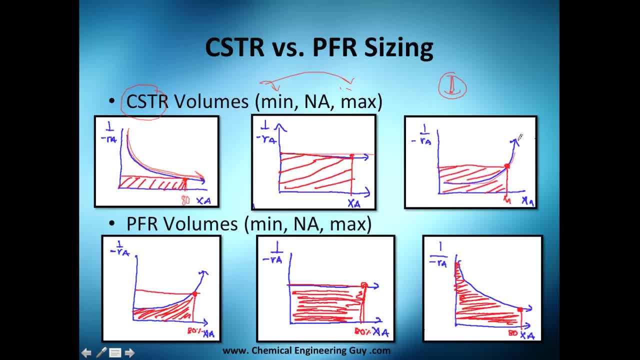 here, it's straight here and it's going upwards. here at eighty percent, you crash with this line and you turn horizontal. this will be your volume. and look that you are not analyzing the area under this curve, which is cool, because then you will need more volume. this case is the- let's say, the. 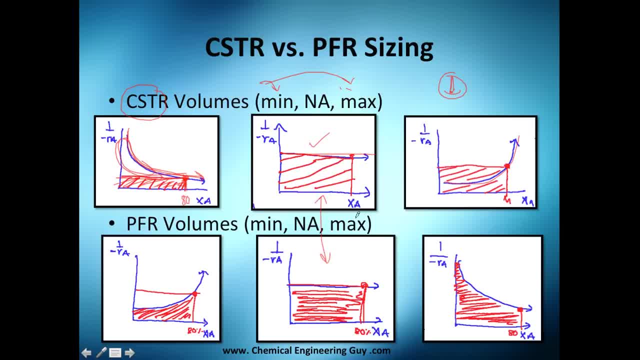 neutral case because it's the same for PFR and the CSTR. you cannot do anything. it's set, you cannot do more and when you have these uh type of rate of reactions, you don't want them because you're going to have these X's here. 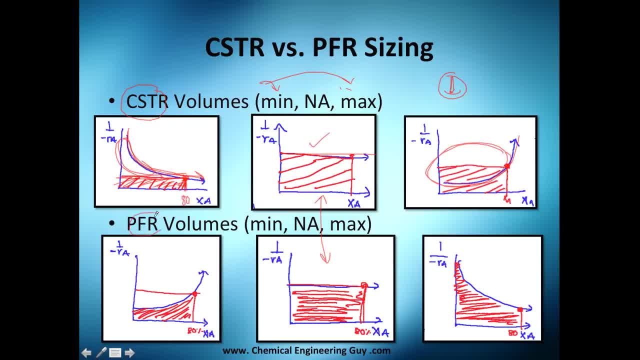 okay, that that is for CSTR. now let's go for PFR. I also order it from minimum volume to maximum volume and look how they invert the same type rate of reaction. but this time we are not using this volume here. look, this is empty. we are using only the area under this curve, which is cool. so probably if you have this, 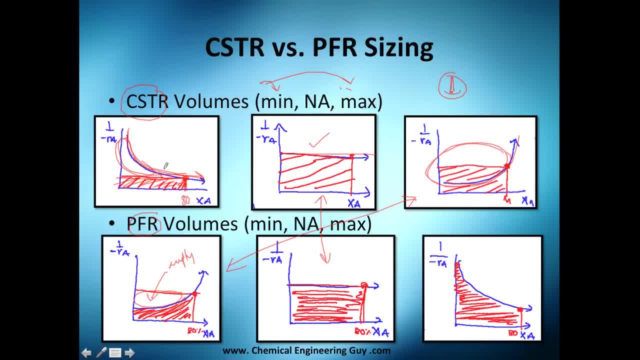 reaction. please choose a pfr. you have a reaction like this. you will see that if you were having a CSTR, you will not be using this volume right here. so CSTR will be nice here and CSTR will be nice here. so just take that into consideration. don't learn it by heart. 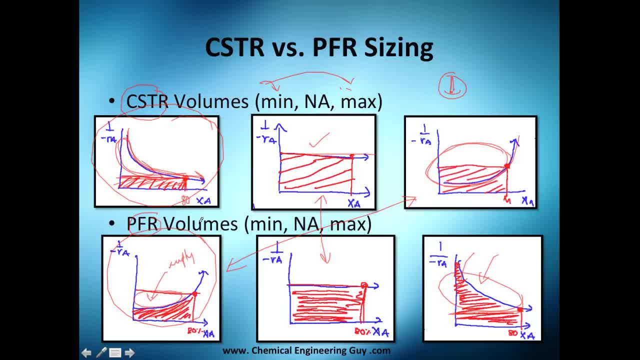 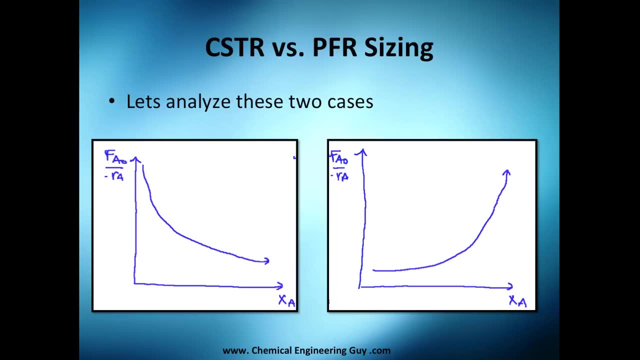 learn it by a definition of CSTR is always the algebraic, let's say mathematic, form to get it, and PFR is the integral mathematic way to get the volume. and this is what I was telling you guys: the one that goes decreasing and the other one that goes increasing. 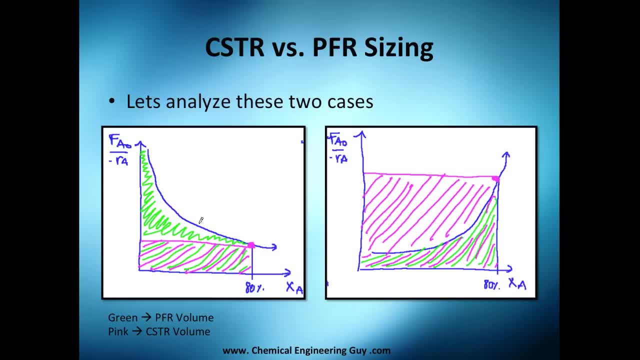 let's analyze both cases. same story I told you before. the green one is PFR. so when you have these type of rates, you don't want PFR because you're going to have these X's. this is the least volume you will need for either reactor. so 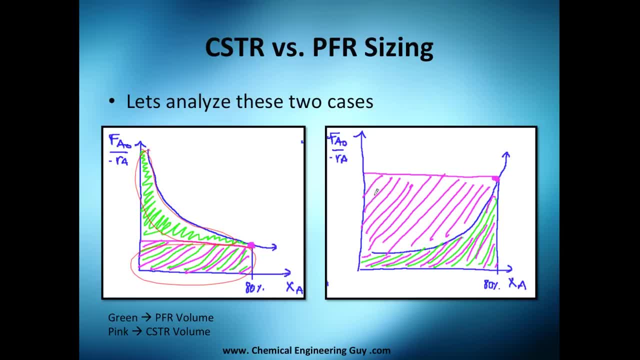 you will choose a CSTR. it's the minimum volume you will have now if you have an increasing rate of reaction. look all. if you were to choose a CSTR, you will have all this wasted away. I think CSTR will be worst. so a good guess is always. 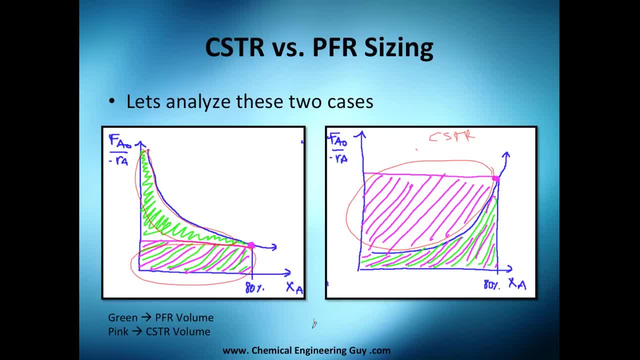 if you have no idea of the rate of reaction, choose a PFR. maybe odds are that it's almost 50-50,. if it is a decreasing like this one, you will be not that bad as if you choose a CSTR. but if you choose this one, the odds that you 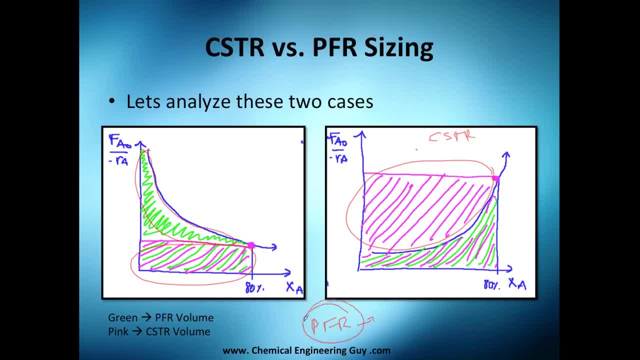 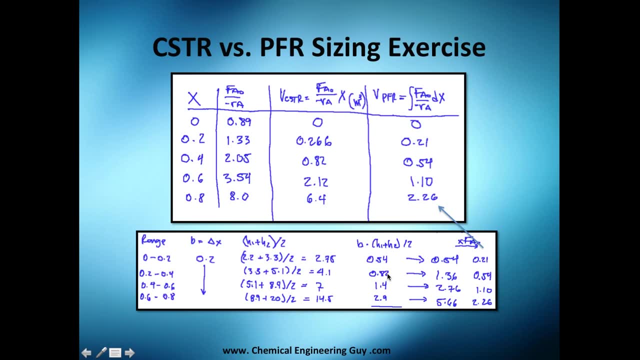 get better are way better. so I would choose always. if I had no clue, I would say PFR in general will give me the least volume and I'm going to do this exercise, but I think I'm going to split it in another video, so see you.